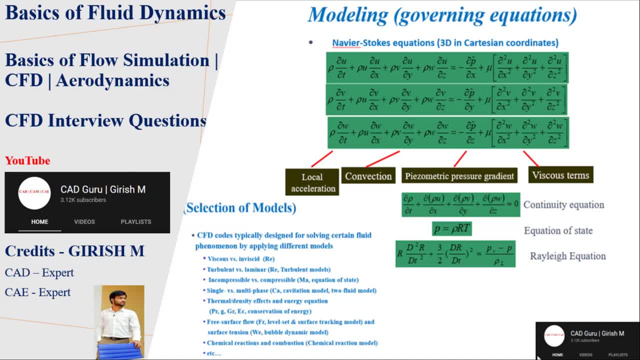 Hello everyone, myself Kirish with basics of flow simulation, CFT and aerodynamics. So this content, I have just gathered it from the internet. Okay, it's for educational purpose. Well, we'll see what and all the basics needed for fluid dynamics as a picking up. 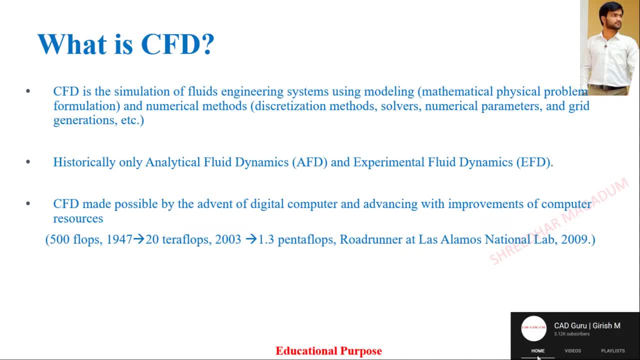 What is CFT? It's a computational fluid dynamics which will help us to deal with the simulation of fluid engineering systems by using modeling and the numerical methods. Okay, and numerical methods? we can say: first we'll describe or discretize the model and then we'll use the 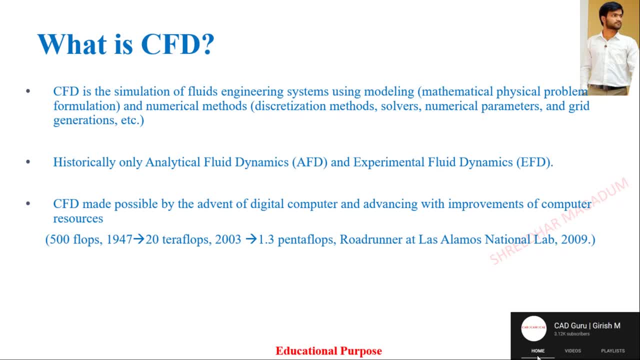 solvers and numerical parameters. By just doing the grid generation we'll get the outputs Okay. there are two types of like CFT analysis. One is EFT and EFT, that is, analytical fluid dynamics and experimental fluid dynamics. So during 1947, we had 20,. 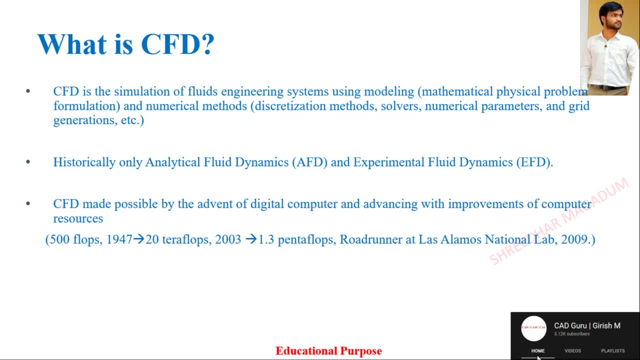 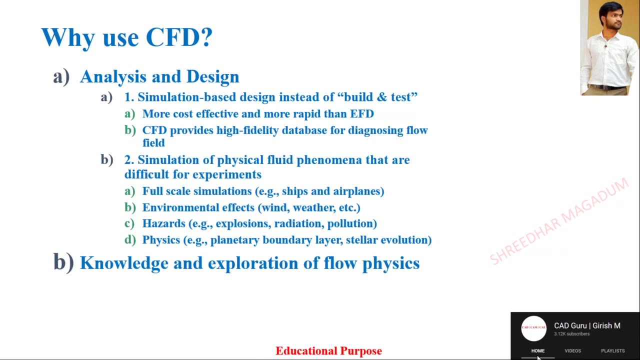 teraflops and then, during 2003,, we have 1.3 pentaflops. Okay, so these are the computer resources, and then it keeps on increasing year by year, Why CFT is needed. Okay, so if you are going to analyze and design based on the like aerodynamic, 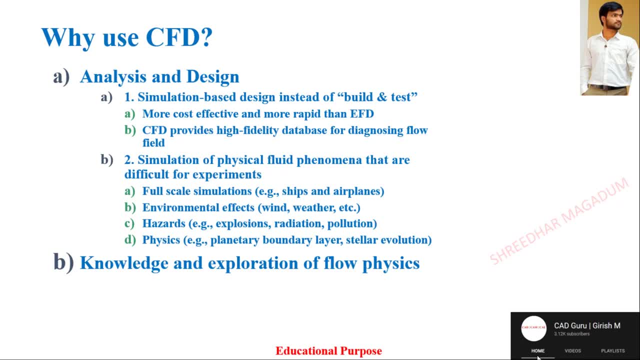 dynamics called as on ships and airplanes, like environmental effects, like winds and weather, and if I consider hazards like explosions, radiations and pollutions. So in these all the criterias, we do use the physical fluid phenomena. Okay, that time. 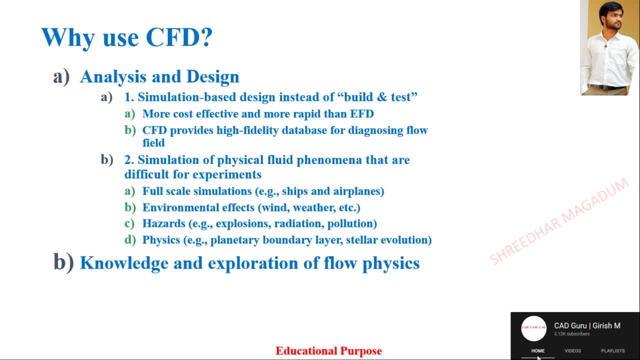 it is very difficult to deal with the experimental methods, So that time we use it, Okay. And then to get to know about the exploration of the flow physics, Okay. to gather the knowledge of what, the how the flows will happen And what are the physics behind it. To just deal. 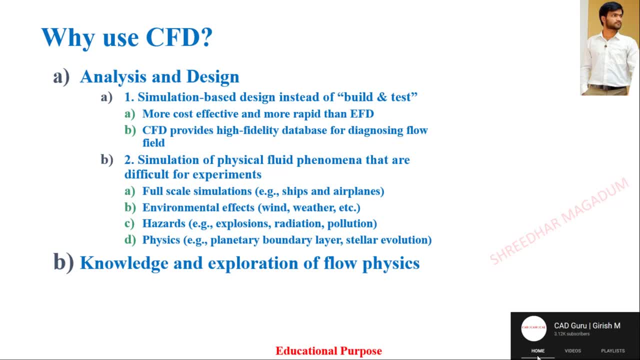 with these all the steps, we use CFT. Okay, there are different sub domains as well. So, like external analysis, internal, and we even you can consider the HVAC analysis and the. then if I consider electric cooling and then comes with aerodynamics, like that is finding. 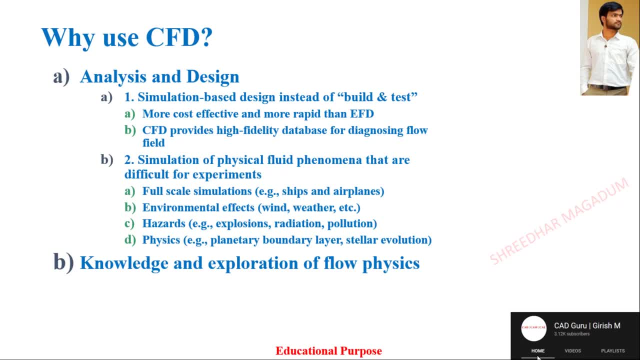 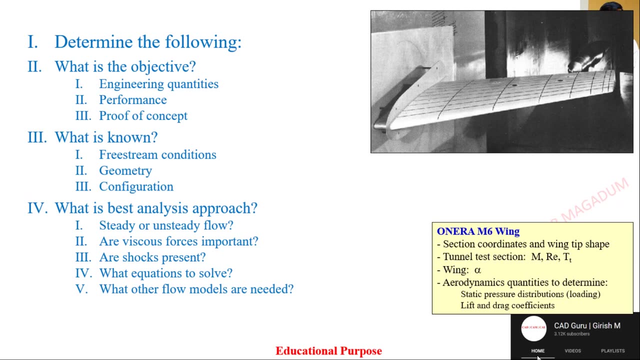 out the coefficient of lift and drag and finding out the vorticity turbulence. these all the things will come into account when you are dealing with the CFD. So before starting with the CFD, we need to know what exactly we needs to do first thing. 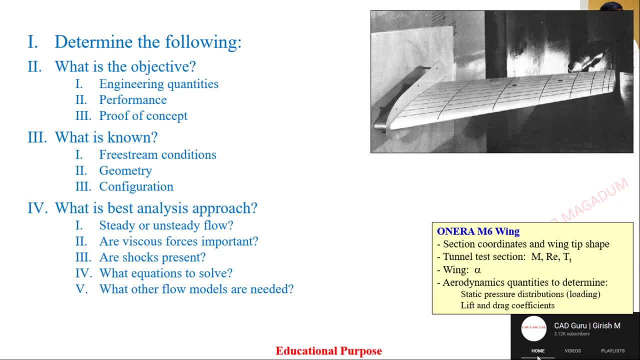 is to cross check what exactly the objective is. so what we are looking for. so proof of the concept, the performance and the engineering part, it is ok. what should we know? the free stream conditions: ok, and then geometry we need and the configurations: ok. what is the best analysis approach, what exactly we need to follow to deal with the analysis? ok, first, 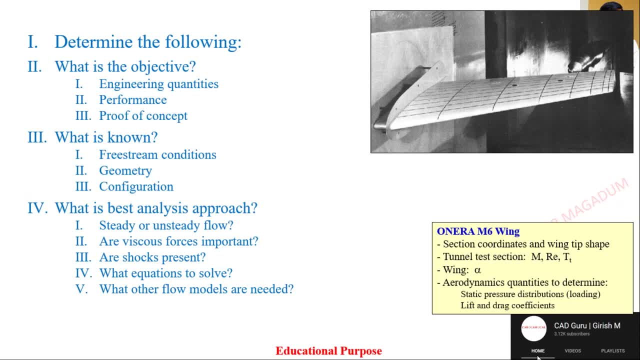 we need to Check which type of flow. it is: steady or unsteady, right? is there any viscous effects into it, or whether the shocks will be present or not. so which type of equations we need to choose: iterative or something else? ok, and what are the flow? models are needed. ok, these: 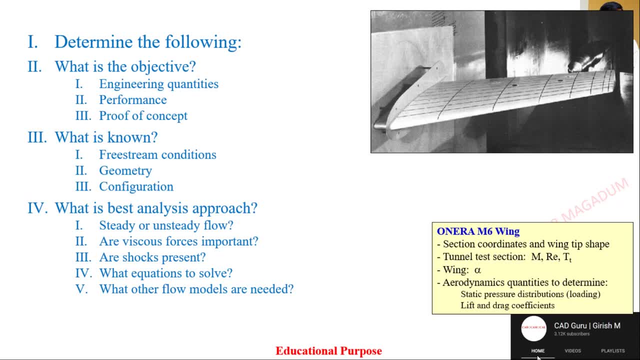 are the things we need to consider. So here the simple example, that is Practically Practical testing, experimental testing, that is like wind tunnel testing. ok, the airfoil section has been taken with that, we will just cross check how exactly the aerodynamic quantities will change. ok, that is lift and drag coefficients and static pressure distributions. this is 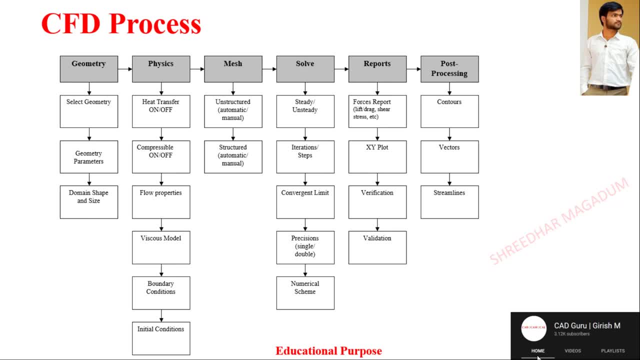 a simple flow chart which will explain what exactly will go through the step by step process. the first thing is geometry, Where in we just select geometry and we will define the geometry parameters. we will simplify the geometry over there and the domain shape how should be the computation domain we need? 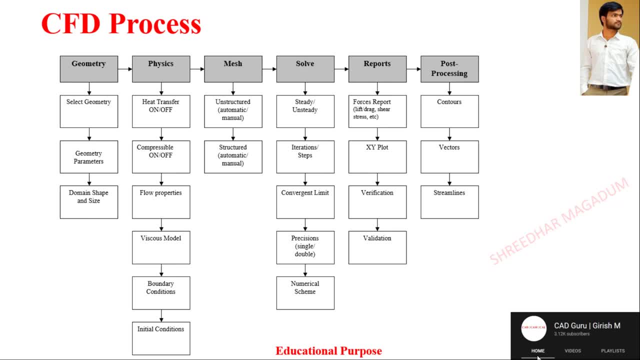 to select and what is the size of it and how much size we need to consider and geometry conditions. ok, coming to the physics, we will cross check whether we need to include the heat transfer in solids or not. ok, on or off. compressible or incompressible flow properties. 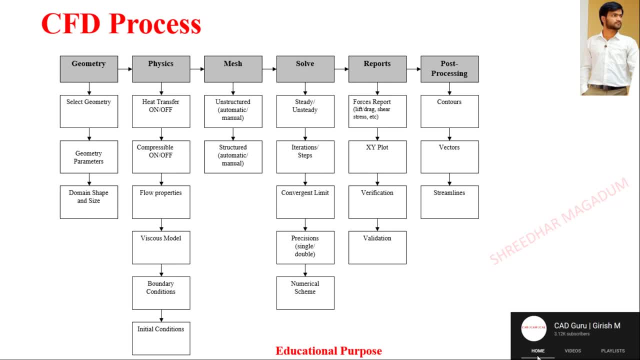 like turbulence or transition. So this is the first thing we need to consider: Ok, Ok, Precision flow or Super Sonic flat block like this, with respect to, and also where we can, him and Larry, Ok, Viscous or Inve baked low. 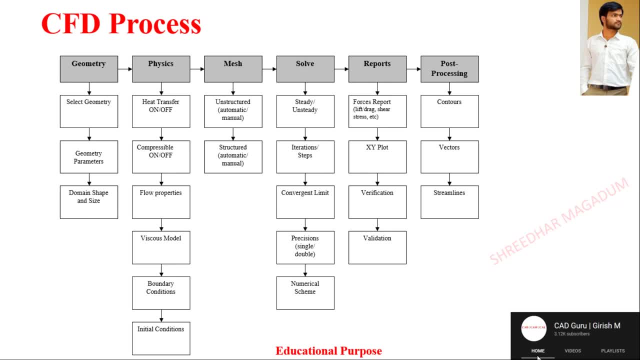 Bond conditions, like what exactly the inlet and outlet pro are working as pressure of the outlet, like this, ok. And initial conditions, feelartenish condition, like room temperature. what is it ok should be flu growth medium, which you are taking into account. artisanي should be lost at your. 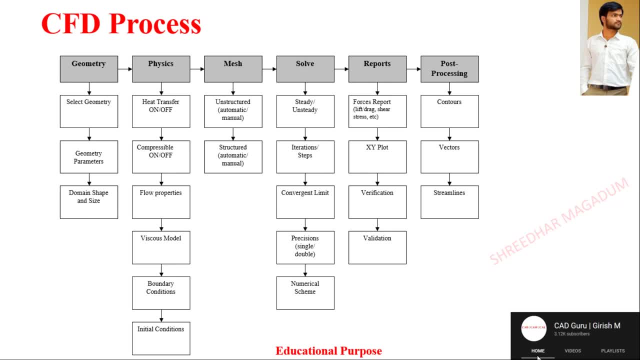 foot Thinks. Coming to the mesh, There are two types. one is structured mesh and unstructured mesh, automatic and manual, depending upon the quant. you can just measure: solver, steady or unsteady iteration steps. okay, now convergent limits. so which value you want to converge, as you will stress or question? 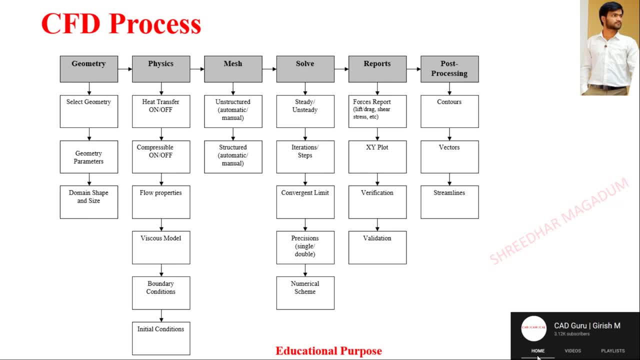 of lift or drag, like that. you can consider precision, single audible precision, and this will be explaining during the answer sessions. remember this one. okay, then, considering the outputs, we have the reports according to that, like XY flots and lift, drag, shear stress flots and then verification flots, and 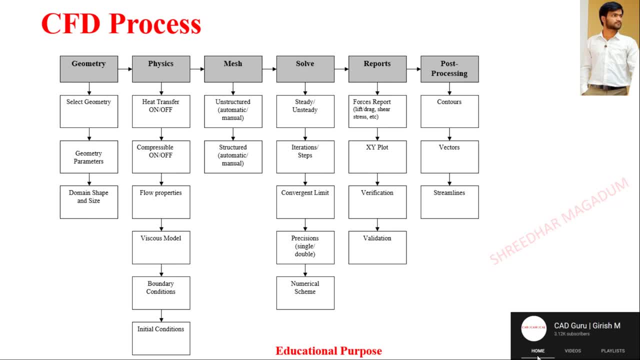 all you can just plot it up. once you get the results, post processing, you can just use the counter flots like temperature, flot, velocity, flot, pressure, flots like this and even mass fractions, and all you can include the multiple of counters, actually now vectors- how exactly the flow is happening, with vertices taking place. 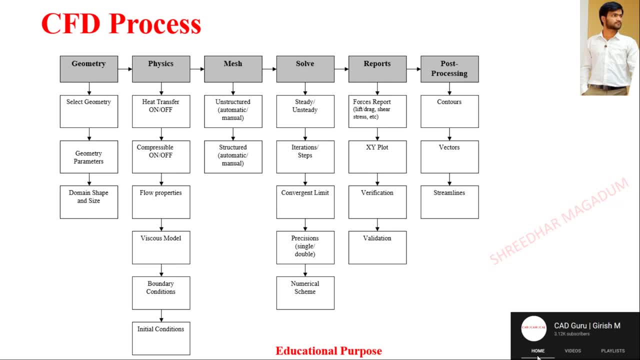 these things. to find out, you can use the vector flots streamlines- how exactly the flow is happening. okay, and by just visualizing the streamlines we could able to just optimize the results or optimize the design pages, cross checking the same. okay, so this is a short explanation about the entire flow chart. 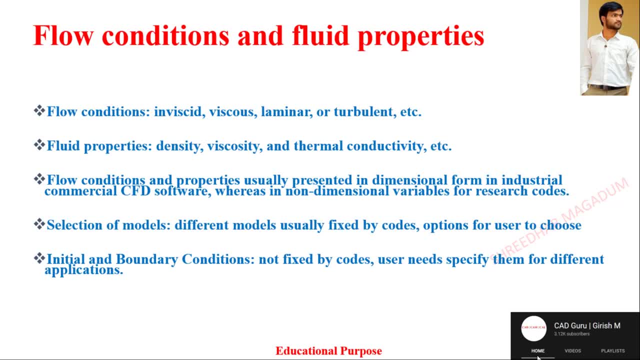 of the CFD process. coming to the flow conditions and the fluid process. so if I consider flow conditions, we need to know about the inviscid, viscous, laminar, turbulent flows as well. okay, if I consider the fluid properties, we need to know the density of the fluid viscosity and the thermal conduct here at that. 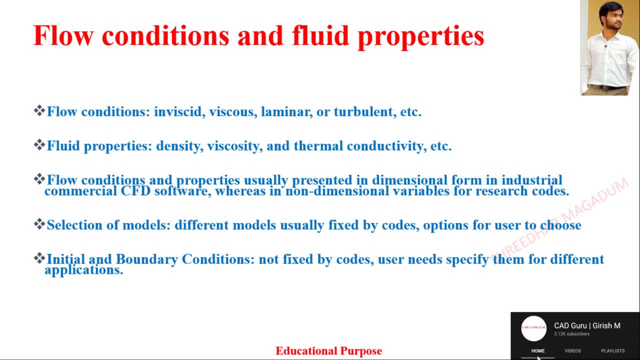 particular flow which we are considering. next, the selection of models, so there might be different models available. so which model we need to choose? okay, there are fixed course available for that and initial boundary conditions. like what exactly we need to define the initial conditions that we all need to crochet? 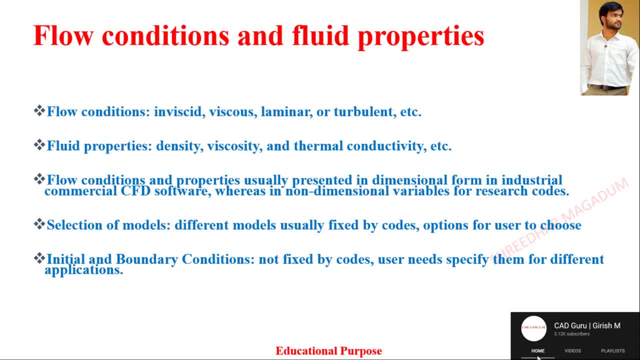 these or the things? okay, so which software also they need to use? that is also very important. there are so many softwares available in the market. which is the best run and which I need to choose. with respect to caustings, okay weather if I choose the multiple software, so if I choose the lowest cost. 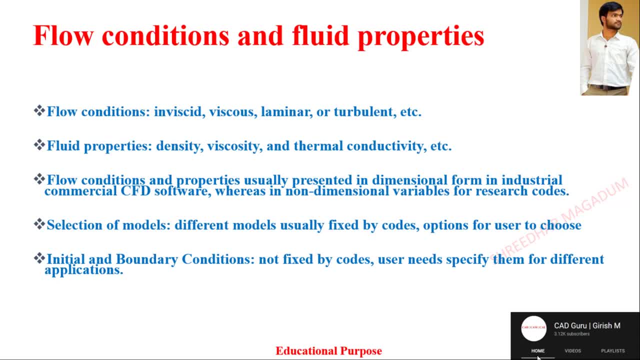 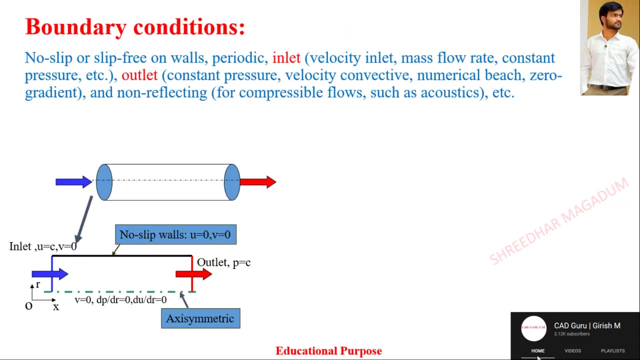 to give the results with respect to higher software or not, like that, if we can cross check. but depending on the pricing, the standards, the capabilities will vary. but if you are looking into specific condition might be same everywhere. remember that. yep, coming to the boundary conditions. so here you could see the inlet and outlet conditions we have defined. so with respect to that, 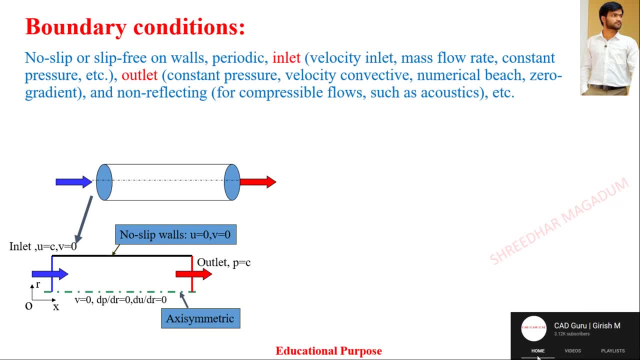 if I consider inlet, they might be slip or they might be free conditions on walls- okay, in that, like velocity I can define mass flow rate and the constant pressure I can define as some boundary conditions for inlet- okay, and outlet, constant pressure, the numerical beach and zero gradients and all. and if you are considering the non-reflective. 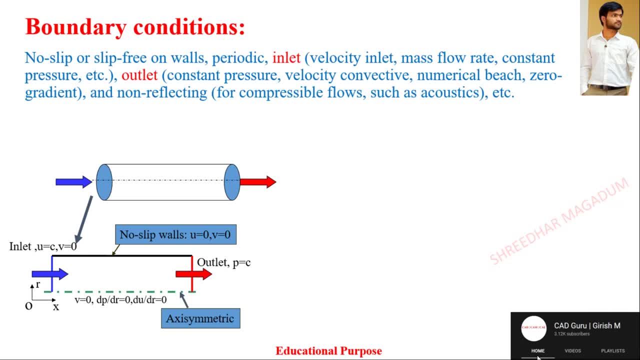 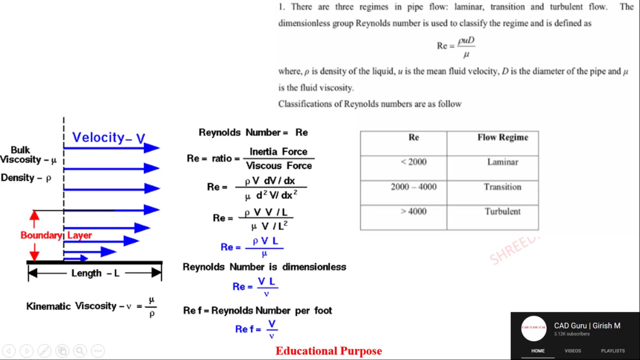 components of the fluid, okay, decompressible flows and, if you want to include the ecostics as well, so these things again take into account, okay. so this is the simple explanation. the viscosity effects, okay, and reynolds number: so what exactly the reynolds number? so why we use it. 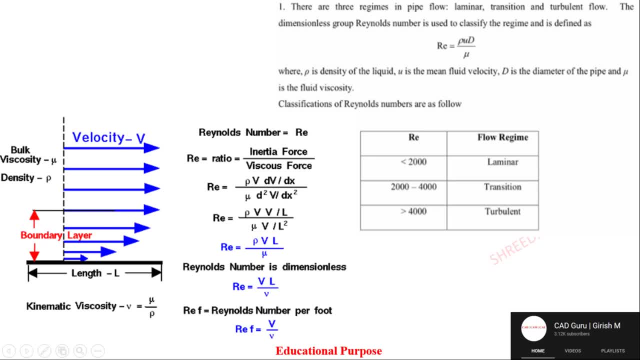 to just give the classifications in the flow, that is, whether the flow is laminar or the turbulent or that is transition phase, how we can predict by using the reynolds number formula, that is, rho, vd by mu, where d is the diameter of the pipe and u is the fluid velocity. 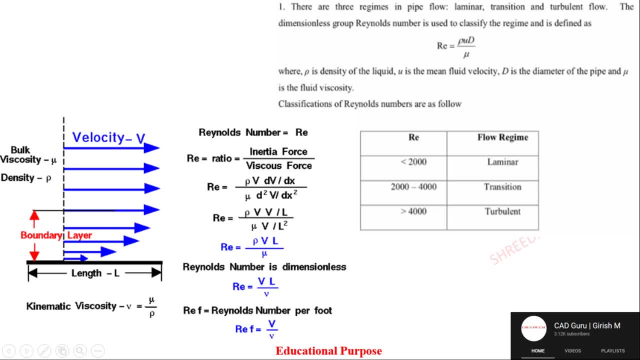 rho v velocity. so if i consider the density of the fluid is rho and mu is the uh viscosity, we can say dynamic viscosity. so you could see this is the excurs force and the reynolds number. so if i consider the reynolds number, less than two thousand. 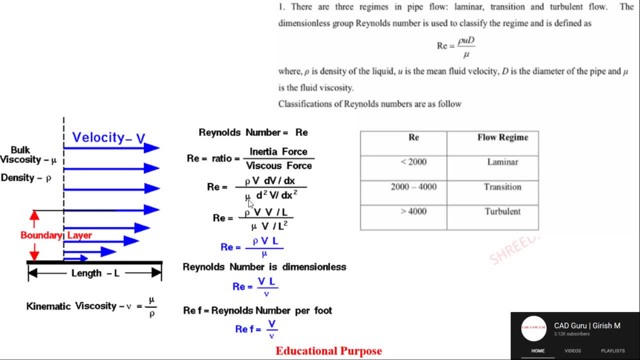 we need to consider that as a laminar flow if you're considering transition two to four thousand and turbulent more than two thousand four thousand. so uh, while defining the uh, this parameter will keep it automatic. sometimes, if you know the reynolds number, you can choose whichever you want. 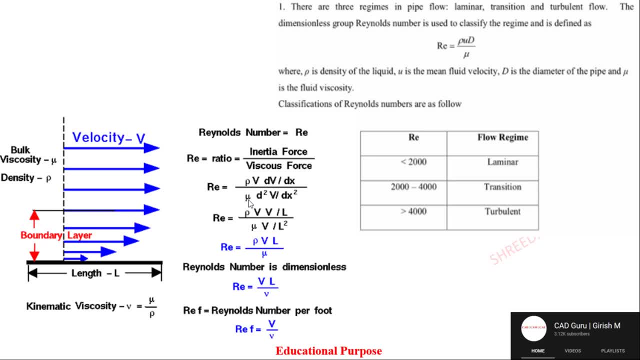 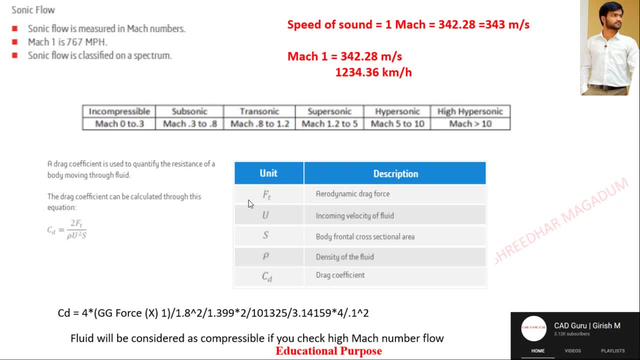 okay, software is capable of knowing which exactly we need to choose. uh, coming to the speed of sound, we already know it is three forty three, that is, one, two, three, four kilometers per hour. so i'm weak with conversations speed, which is a good distance by time. 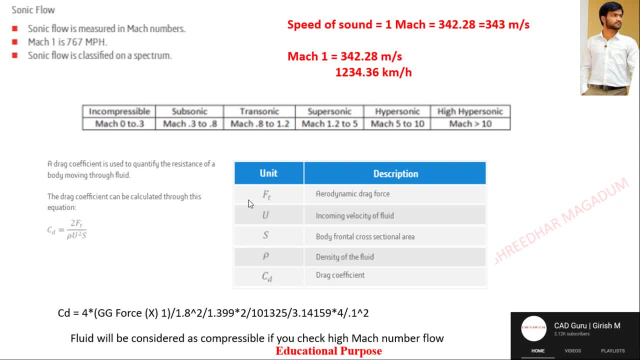 this formula i use and then i can convert two meters per second to kilometers per hour. remember these things. so speed of sound, which is equal to one mark. so the flows will be just measured in terms of subsonic transition, supersonic flow, hypersonic flow, depending upon the mark number. 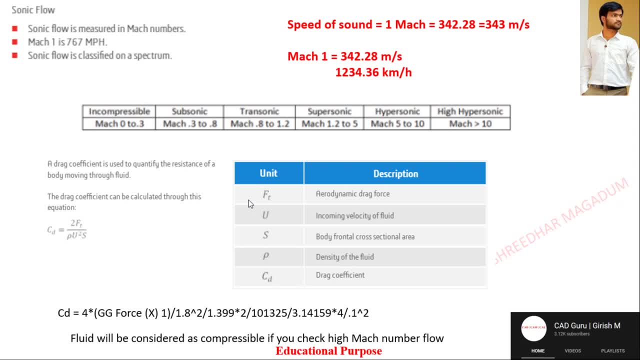 that is one mark which is equal to one, two, three, four kilometers per hour. okay, thousand two hundred and thirty four. supersonic, you already seen, we have the aircrafts: fighter aircrafts, according to that, teachers, if i consider. and then, uh, we have different aircrafts according to that, the supersonic or hypersonic. fighter aircrafts as well. we have. okay. so the classification, if i consider subsonic, it is, it should be a point three to point eight and transonic point eight to one point two, and then, if i consider supersonic one point two, two, four or five, you can consider, or more than five- it is hypersonic- or more than. 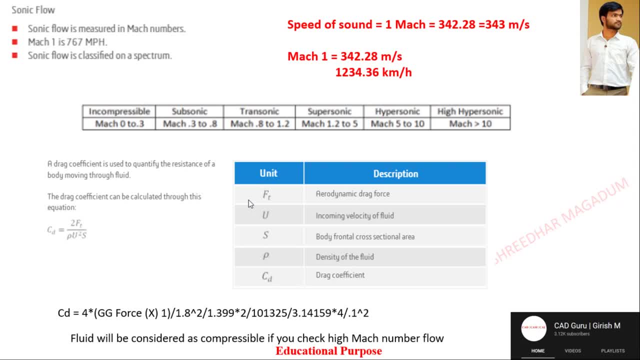 four, it is hypersonic sometimes, okay, uh, talking about coefficient of left and coefficient of track. so how you gonna calculate this one? so, if i consider solid works flow simulation, you will get the lift and drag first. according to that, you can formulate the equations to get the coefficient of lift and drag. okay, the formula is coefficient of lift, which is equal to two times of lift divided by rho into v, square into s, where s is the frontal area, not overall area. very important factors needs to be remembered. okay, if you are going to insert the equations dealing with this one, you need to remember the 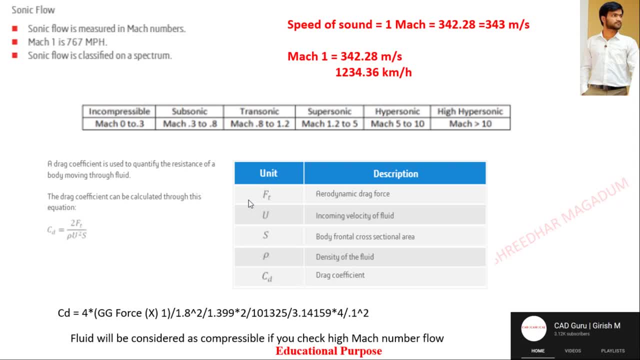 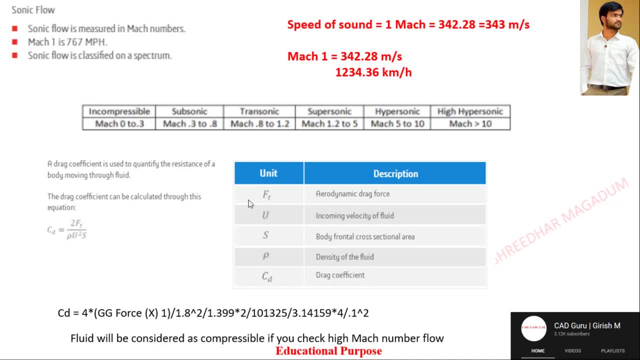 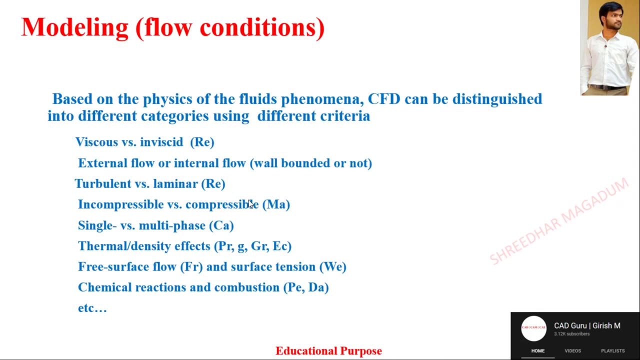 if i implement the formula cd, which is equal to four times of gc, into uh, that is, drag force and then velocity, squared this formula, okay, fine. so this is all with this modeling. if i consider modeling, we need to cross check based on the physics of the fluid phenomenon. uh, we'll just use the c of t. 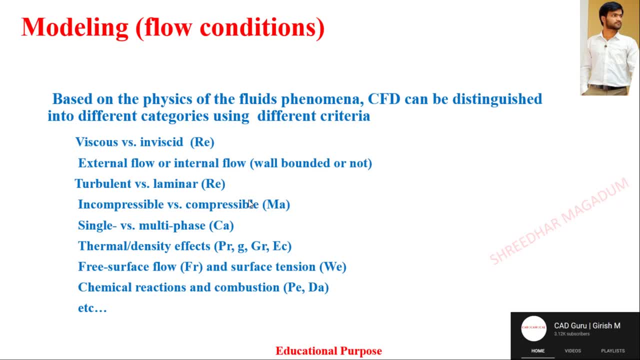 to just categorize the c, that is viscous or inviscid, that is depending upon the r-e, and then laminar and turbulent pronounced number, again like external internal flow, and then compressible, incompressible, a single or multi-phase and free surface or surface tension is included. on what we need to cross check. 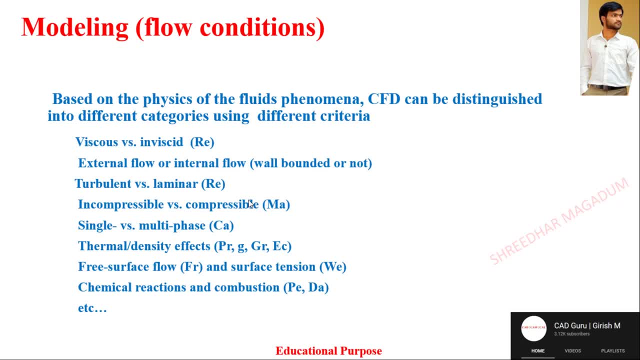 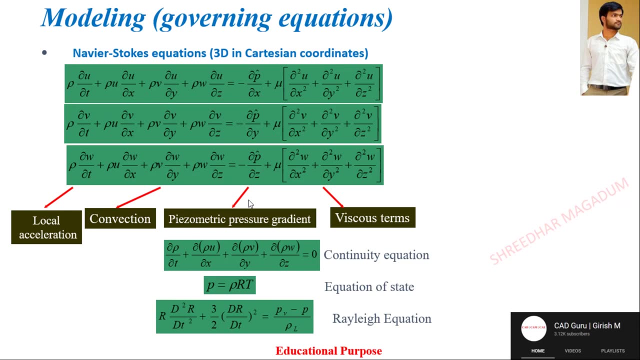 okay, chemical reactions and the conditions: is they taking place or not? these things they need to first check. so we'll have a few expression about these all. the term, the Navier-Stokes equation: this is the entire equation, very important equation. okay, it looks complex, but all the CFD modules will refer this. 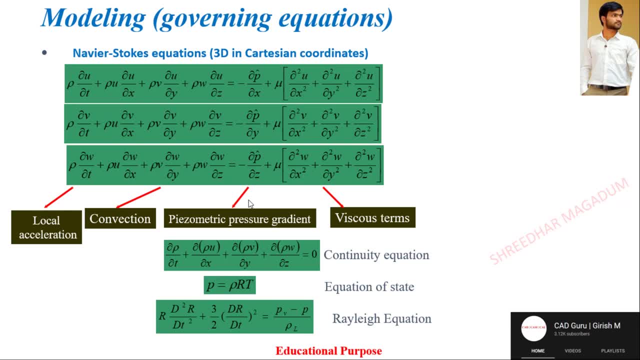 one as a reference. the things are like: we gonna just utilize the continuity equation and the equation of states and the Ray equations to solve the safety equations. okay, you can see viscous jumps. so at this location. if it is so, it is on this equation. so if 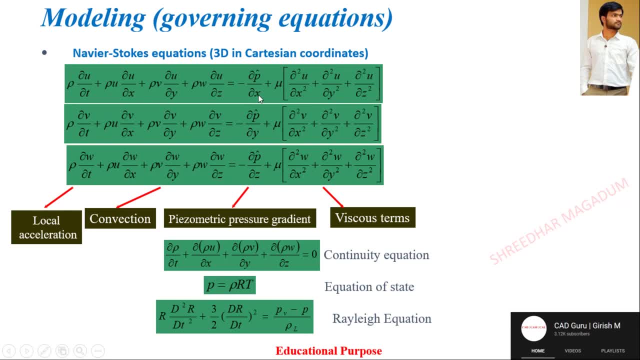 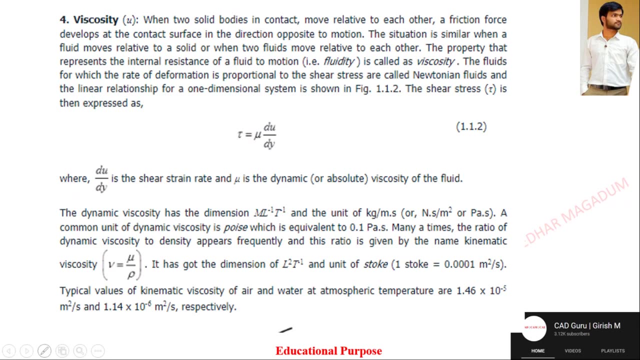 I consider, in the pressure gradients you want to deal with this one, or conversion-conversion, and the radiation is considered and thus equation will be solved and if you going to take the local acceleration, so this will be into account. okay, viscosity: so we already know what exactly the viscosity is, if it is the resistance. 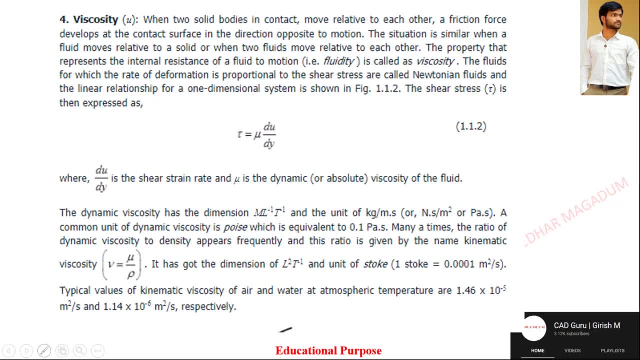 to the flow of any of the fluid over the another layer of the fluid. okay, that is shear stress, if I consider shear stress, which is equal to shear us, if I can stress by strain, which is equal to. let me just see the formula, if I can. so, if I. 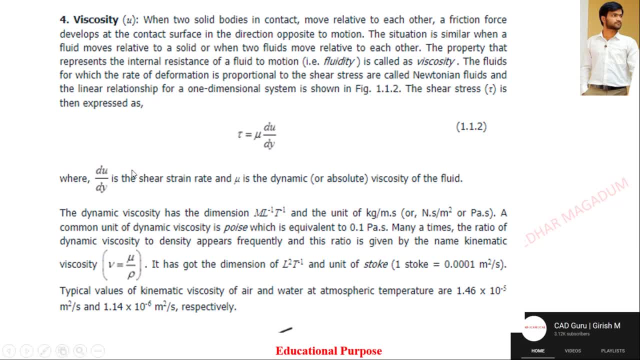 consider here it is shear strain he has taken, that is stress by strain, which is equal to dynamic viscosity. formula: okay, shear stress by shear strain is dynamic viscosity. again, if you are considering dynamic viscosity, the formula is this: okay, and then the expression you could see. I can consider one stroke, what exactly? 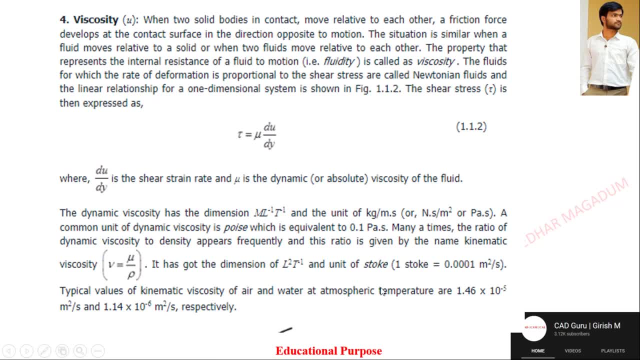 the value is 0.001 meter square per seconds, and again, few things. dynamic, sorry, kinematic viscosity of air and water is given here: 1.46 into ten to the minus 5, 1.14 into 10 to the minus 6. you don't need to remember these all the. 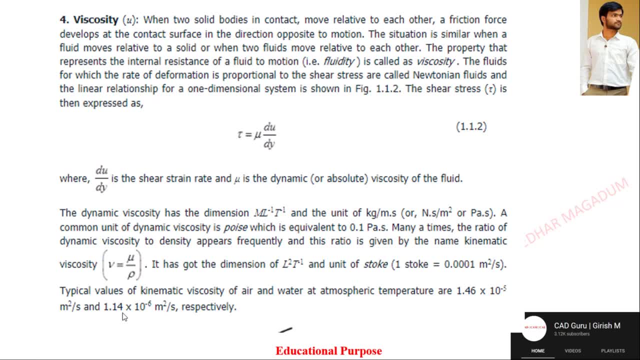 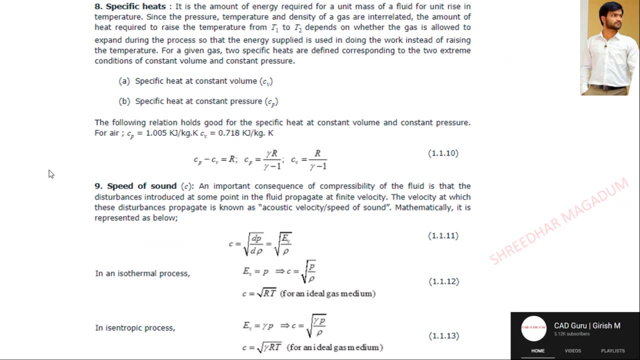 steps because, anyway, if you google it you'll get it, okay. so if I consider the dynamic viscosity in poise, it is equal to 2.1 Pascal second: okay, fine, so you, this is all about the viscosity. if I consider the specific heat, the amount of 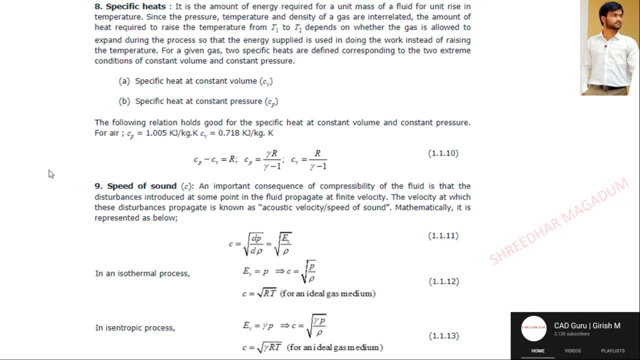 energy, okay, required to raise unit mass of a fluid for a unit raise in the temperature. okay, so energy required to a mass that is a unit mass of fluid to raise the temperature of in it. that is unit raise in temperature if I consider any of the fluid. okay, the unit mass of that fluid. if you want to raise the 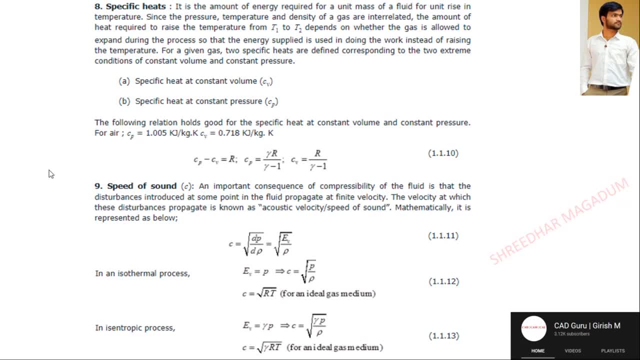 temperature to a unit value. so that is known as the specific heat, the amount of energy. okay, the reason: temperature might be T 2 minus T 1, or the T 1, T 2. we can consider the highest and lowest temperature. okay, so this specific heat has the two extreme conditions with respect to the 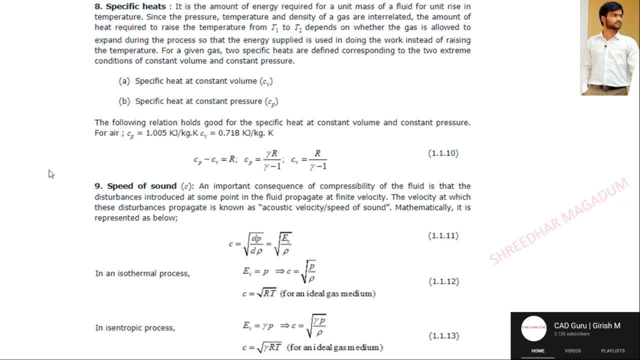 constant volume and with respect to constant pressure, CP and CV. so during engineering we had used these formulas to derive, and these all the equations and the problems related to the specific heat, that is C, which is equal to it is a CP of air and CV of air we have taken. that is CP, which is equal to 1.005 kilojoule per kg. 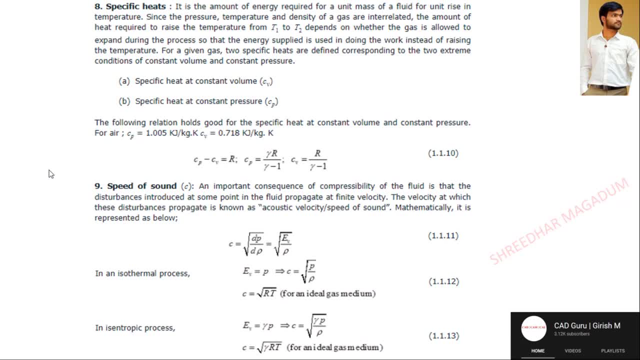 Kelvin CV, which is equal to 0.8, there is 0.718. okay. well, this sound so we already know. so according to that, we can draw the equations. okay, the isotropic process that is C, which is equal to square root of lambda, into RT. 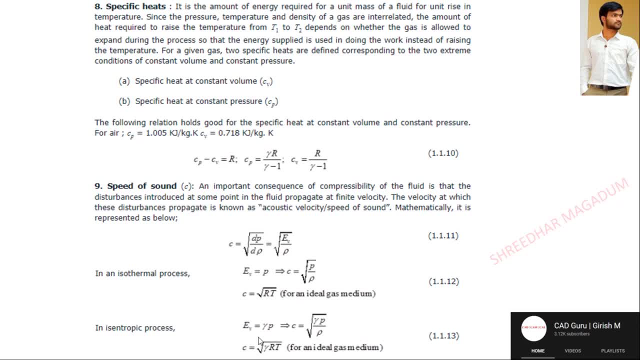 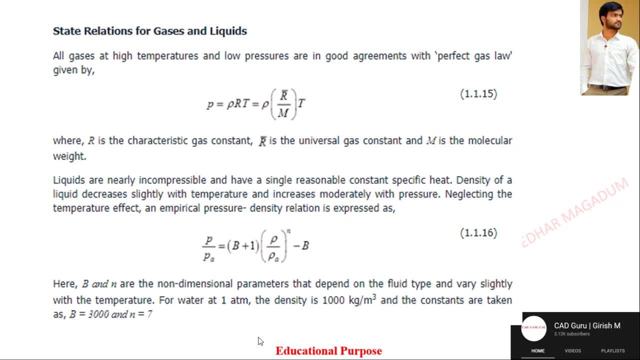 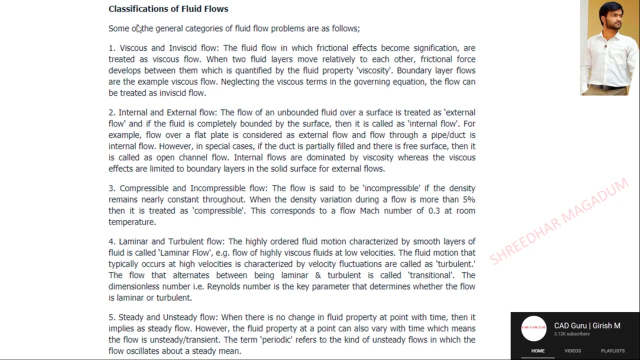 okay, the relations for the gases and liquids. so this is the formula where the perfect gas light is P is equal to row into RT. yeah, you can refer this entire slide to just go through what this perfect gas laws and the expressions, classifications of flows. we have the viscous and inviscid flow. okay, and depending upon the frictional 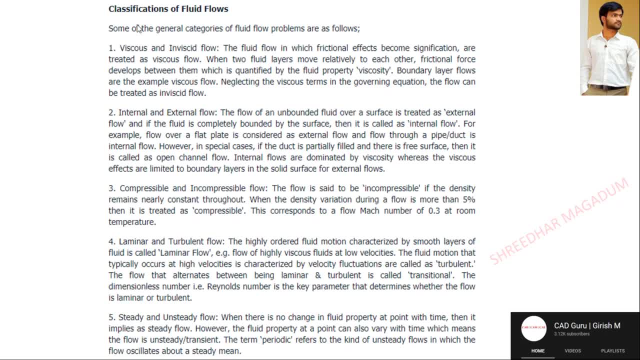 effects. we can consider the viscous or invasive flow and the C flow is calculated in terms of the rate of process and the inviscid flow. okay, and then coming to the internal and external flow, depending upon the internal and external boundary conditions. we'll just go through the. 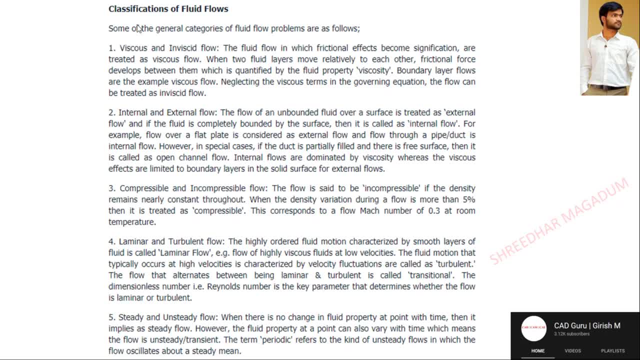 same. okay, if I consider the external flow, what exactly happens over there? the flow of any of the fluid is over the surface. okay, if I consider internal flow, it is completely bonded inside a surface, well, compressible and incompressible flow. so if, if I say any fluid or any, 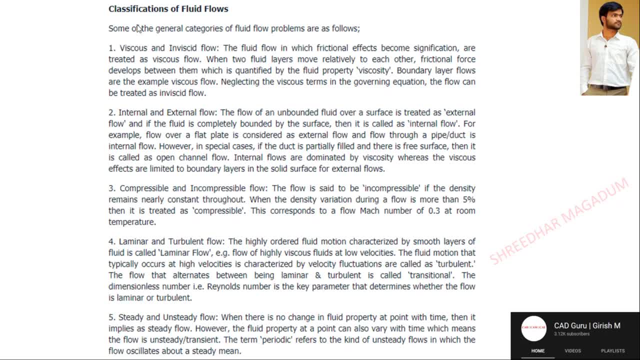 flow which it which is compressible if the density remains nearly constant throughout. okay, that is incompressible. if I consider any of the fluid which can be treated as a compressible where the density variation will takes place, okay, that might be a more than 5%. okay, well, laminar and 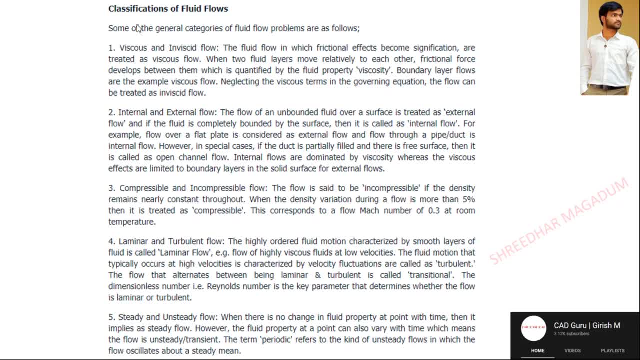 turbulent flows, what exactly it is and how we gonna cross check. okay, if the highly ordered flow motion characterized by the smooth layers of fluid called laminar flow. so I hope you have seen the effects of flow on the airfoil. okay, depending upon the angle of attack, the flow will change to laminar to turbulent, with transition phase as 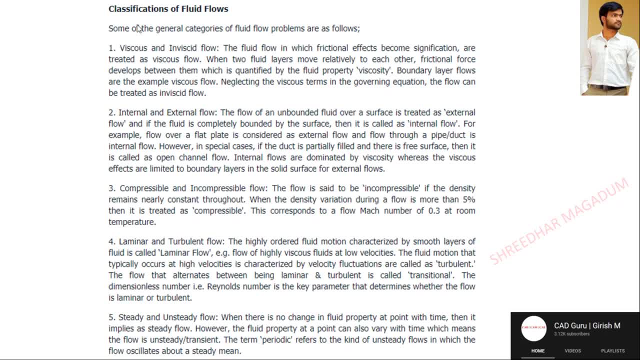 well, okay, for example, if I consider flow with highly viscous fluid at low velocities, okay, that is for laminar flow. okay, what exactly happens with the turbulent flow? the statement: you could see the fluid motion that typically occurs at high velocities. okay, Mach number: we can consider more than two. 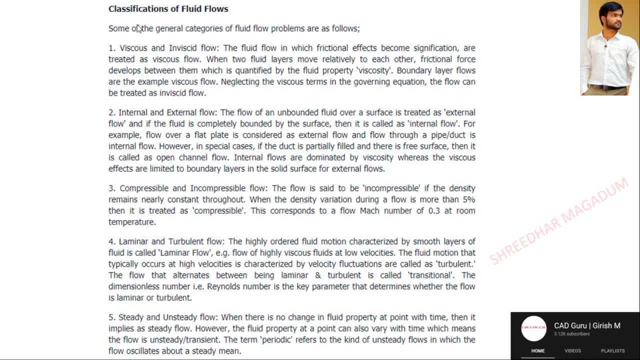 there we can consider the turbulent effects. okay, you can take the airfoil of the circular tube into account and you can start giving the like Mach numbers one, two, three, point, eight, point four and all. according to that, you will get the earth turbulence inside the model. okay, so there you can consider the Reynolds. 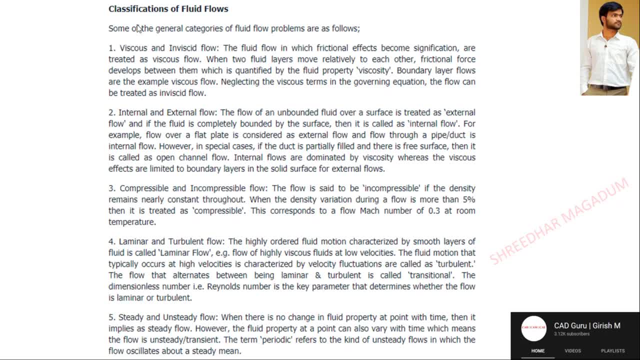 number for the turbulent flow. okay, so that's it for the turbulent flow. okay, so that's it for the turbulent flow. okay, so that's it for the turbulent flow. okay. factor: you can even change the Reynolds number to cross check the same. okay. steady and unsteady flow where there is no change in fluid properties: okay, if I. 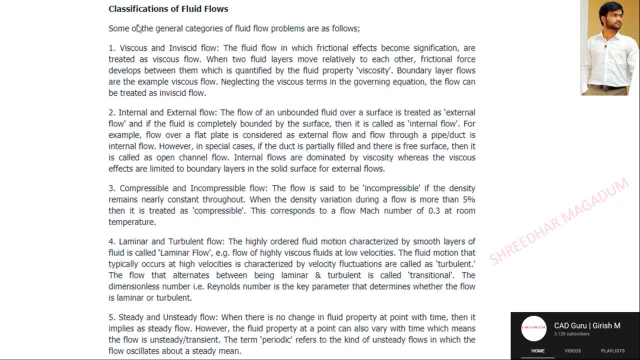 consider steady flow, there shouldn't be any change in the fluid properties at the any point of time. okay, that implies the steady flow, and steady in the sense the flow properties will change with respect to time. okay, remember that. the flow properties will change with respect to time. okay, remember that. 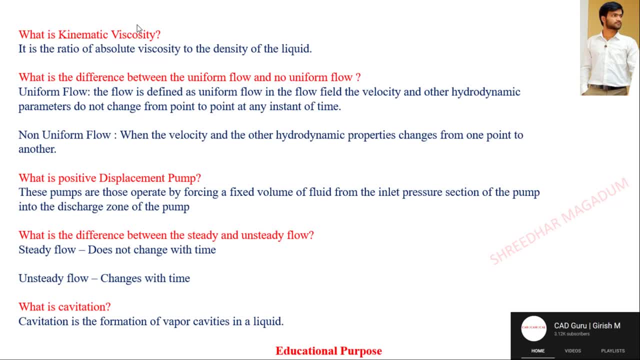 so few of the questions for your knowledge. so what exactly the kind of viscosity is? it is ratio of the absolute velocity to the density of the liquid. so what exactly the difference between the uniform flow and the no uniform flow, that is, non uniform flow, if I consider flow should be uniform, okay, there is a 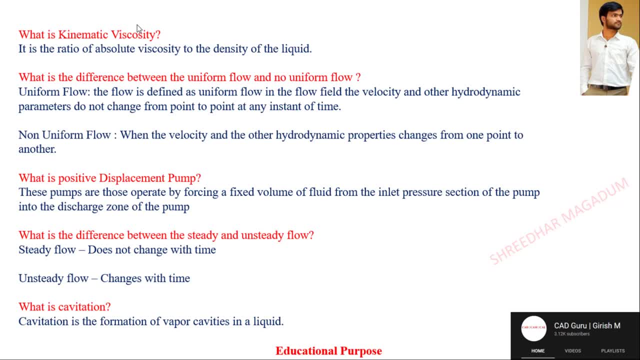 the velocity and the hydrodynamic parameters will not change from point to point in any instant of time. that is uniform flow. the velocity won't change and the hydrodynamic properties also will not change. in non-uniform, in the sense the velocity will also change. Reynolds number will change according to. 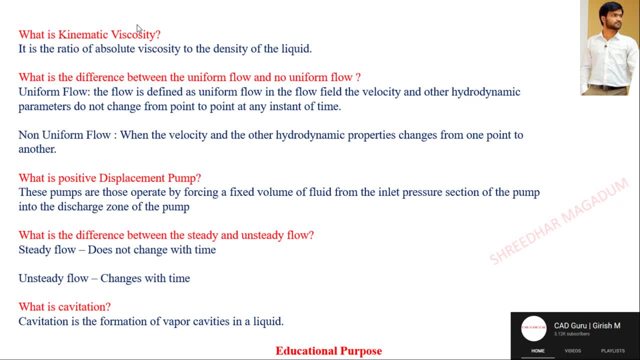 that the hydrodynamic properties will also change. okay, coming to the what is positive displacement pump. so what exactly it means? okay, these pumps are those pumps which operate by forcing a fixed volume of fluid from the inlet. okay, then it will. just what exactly? it is just a minute. these pumps are those operate by forcing a. 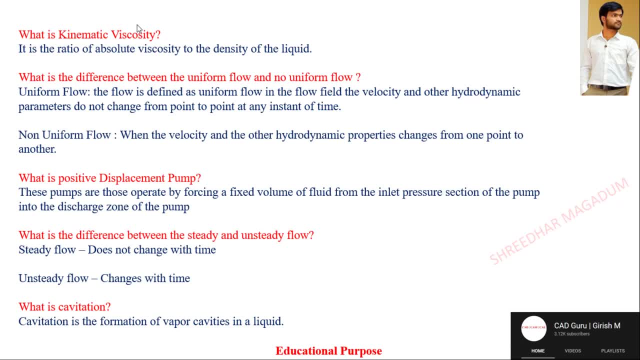 pump which is operating by forcing a fixed volume of fluid from the inlet. okay, then it will just fixed volume of fluid from the inlet pressure: okay. inlet process: suction of the pump into the discharge to zone of the pump, positive displacement. so these will take the fluid. fixed amount of volume. fluid will be taken into the. 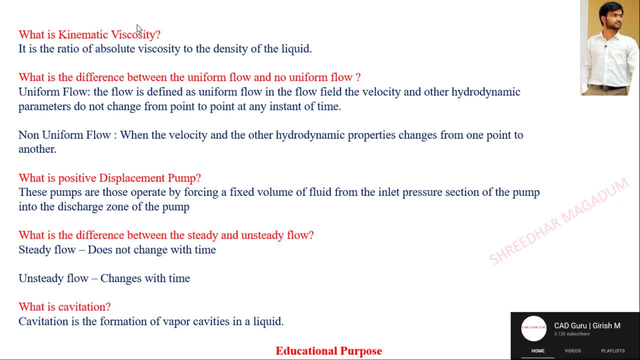 inlet with a certain pressure- okay, inlet pressure- and then thus will be discharged through the outlet. so these are known as the positive displacement pumps. okay, you can just google it accordingly. and then what is the difference between this TD and unsteady flow? as I said, same uniform and non-uniform flow, same thing. the. 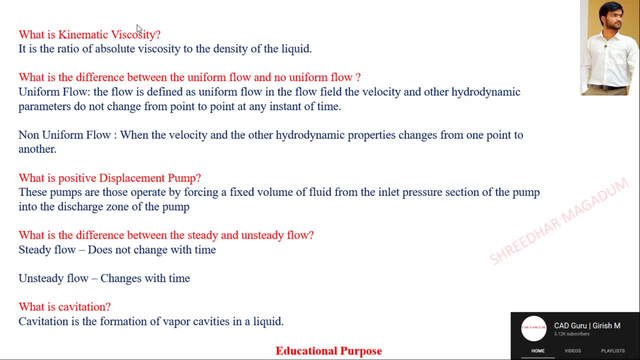 properties do not change with time. here it changes. what is cavitation? okay, the cavitation is the formation of the vapor bubbles. we can say vapor bubbles are the cavities in a liquid known as cavitation. if you want to consider this one, we have the option to include the cavitation inside the CFT or not the pumps, if I 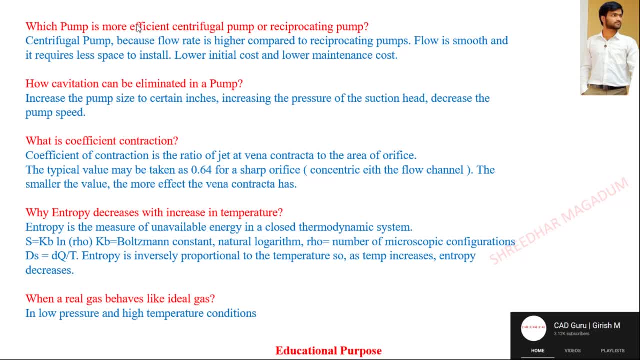 consider pumps. which pump is more efficient? that is centrifugal, our reciprocating last. so the answer is centrifugal pump because the flow rate inside it is higher than the reciprocating pumps. ok, the flow is more there and again it requires less space to install. if I consider the centrifugal, 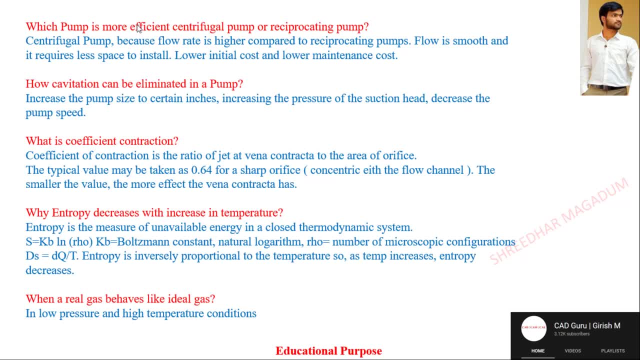 pump and the lower investment cost and the maintenance cost. so how we can avoid the cavitation in the pump? first one: you can increase the pump size to a certain in inches. so it will take a lot of time and research and the development and manufacturing. even you can consider the increase in the pressure of the suction. 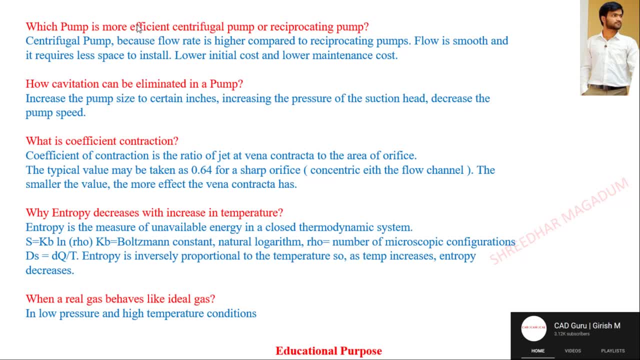 had decreased the speed of the pump. okay, these are the three things you can do to adjust. eliminate the cavitations: okay. what is confident of contraction? it is the ratio of the jet at vena contractor to the area of the orifice, why entropy decreases with increase in. 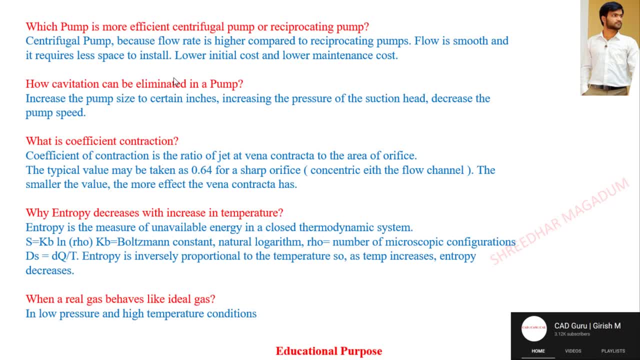 temperature. okay, so we need to know what exactly the intro phase. first see, entropy is the measure of unavailable energy in a closed thermodynamic system. okay, so this, if I consider the formula will be there- that is entropy, which is equal to KB into ln of Rho, where KB is the bourbon constant, and if I consider the Rho, that is the 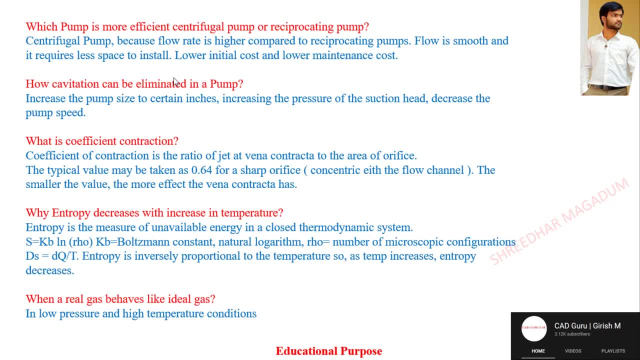 number of microscopic configurations and next the natural algorithm. so the DS by that is discharge DS, which is equal to dq, by T, that is, n drop is inversely proportional to the temperature. by just crossing this equation we could have put you know, as temperature increases, entropy will decrease. if someone asks this question, we can simply counter by: 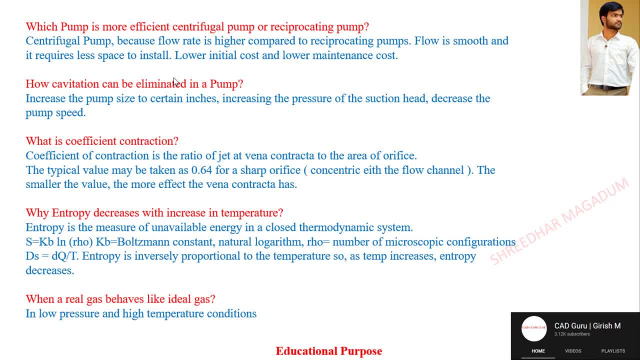 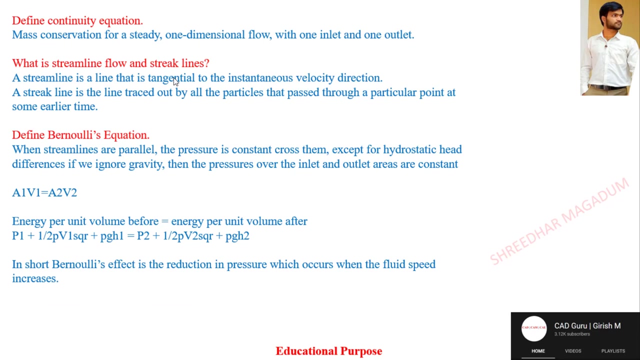 saying: okay, the temperature and the entropy are inversely proportional, when a real gas behaves like ideal gas, when? so? when we consider low pressure and the high temperature into condition, okay, into account. so what is continuity equation? so it is the mass conservation, of our mass conservation for a steady, one-dimensional flow with one inlet and 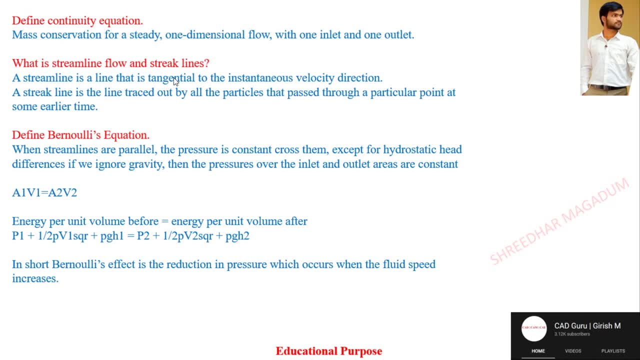 outlet continuity equation. okay, here the mass conservation will takes place. so what is stream line and streak line? sometimes this question plays an important role. so every interviews- this has been asked up to now. we have seen many of the interviews. so streamline is the line that is tangent to the instantaneous velocity direction. okay, 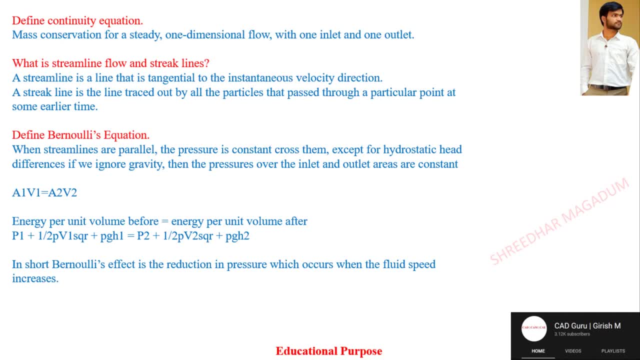 these are the tangential lines which showcase the instantaneous velocity, directions. streak lines is the line traced out by any of the particle, of any of the fluid. we can say, okay, Bernoulli's equation. so when stream lines are parallel, okay then if I consider stream lines, if they are parallel, the pressure. 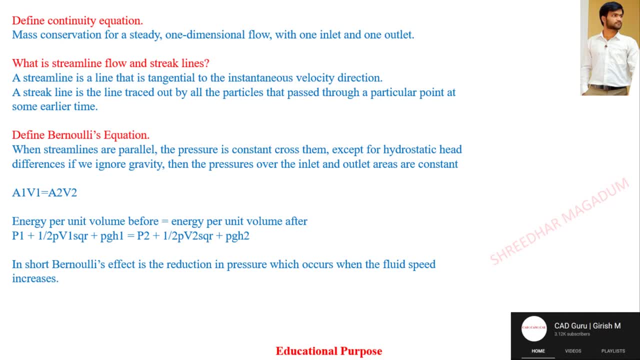 is constant, cross them. okay. and then if I consider, except for hydrostatic head difference, we ignore the gravity, then the pressure over the inlet and outlet areas are constant, okay. and then a1 V 1, which is equal to a2 V 2, we can consider this equation. or if I consider the energy per, 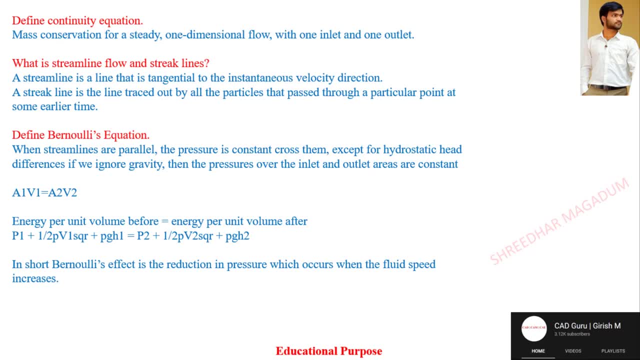 unit volume before and after the flow let an outlet. so it shows the equation that makes v1, last 1 upon 2 row, into V 1 Nas and rho gh1, which is equal to p2, into 1 upon 2 v2 square velocity square. 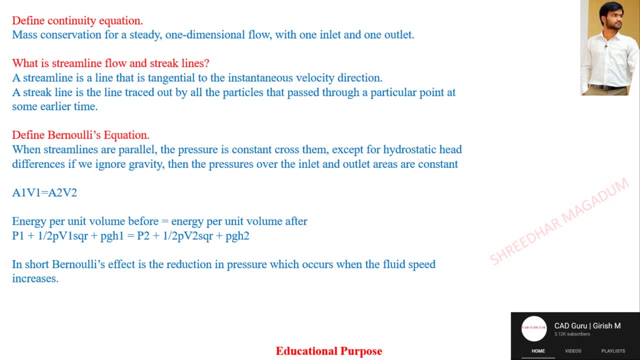 that is rho, actually okay, and then rho gh, square, okay, this is the formula. okay, if i consider in short what exactly the Bernoulli's effect is: okay, it is the reduction in the pressure which occurs when fluid speed increases. okay, the Bernoulli's effect. 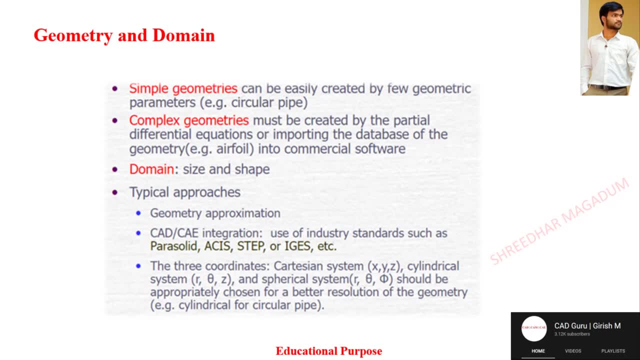 considering the geometry and domain. okay, the simple geometries will be included, like circular pipes, and all complex geometries like airfoils and all we can consider. okay. and then typical approaches by considering the geometry, approximation and the currency integration for consider when it would take the standards, that is, industry standards such as now parasolid. 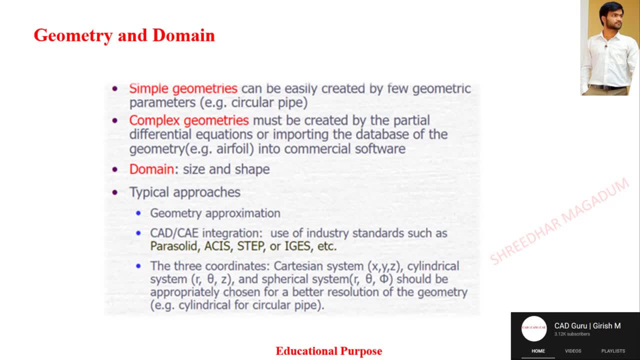 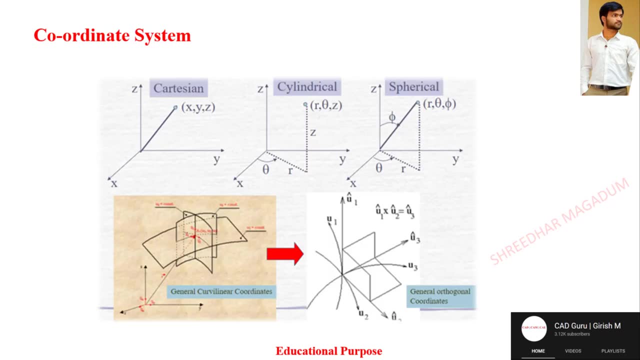 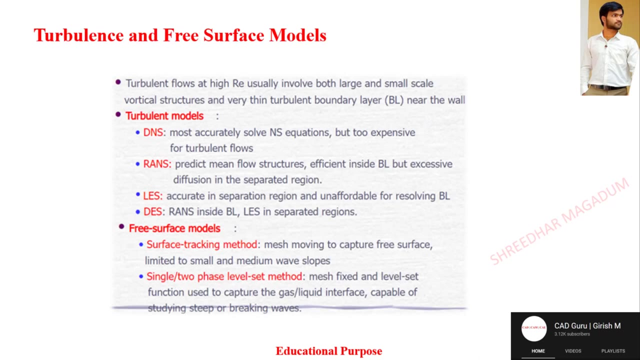 and step files and igs files into account to just deal with this analysis. okay, so there are different types of coordinate systems, that is, cartesian coordinates, cylindrical and the spherical code. okay, depending upon that, we need to define the coordinates. consider the turbulence and the free surface models. so turbulence flows will be you already. 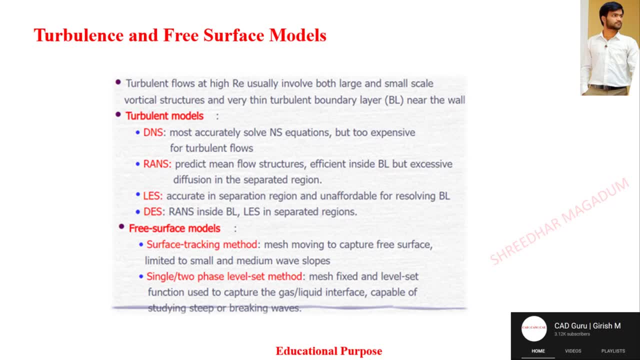 know it is at high Reynolds number. okay, involves the large and small scale sometimes, okay, that is the counter. what are the? it most important unit? it is the. is some other Conclusion. in terms of fluency, your cSt, Austrian superorganisms: okay, there will be a turbulent layer if I consider the boundary conditions. so turbulent models there are, DNS models, realize models to predict the means flow structure. okay, 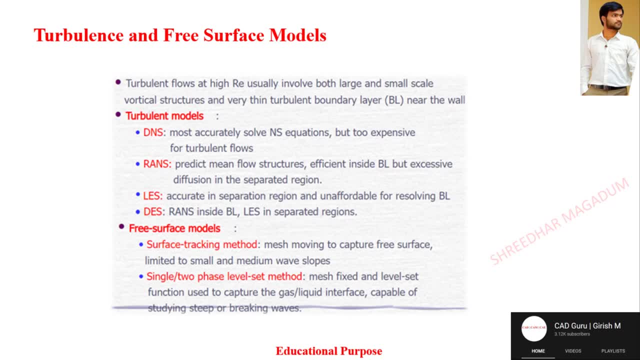 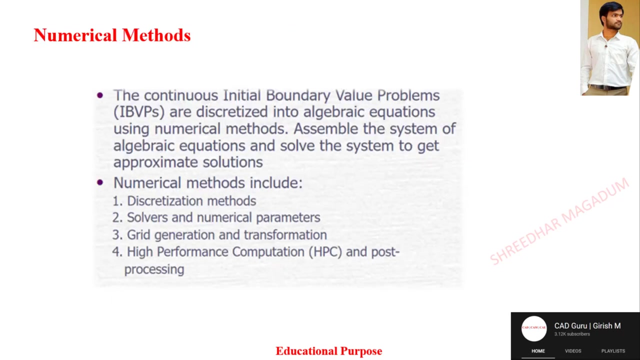 so it is quite expensive. if I consider a DES method where we'll take the RANS inside boundary layer and LES in separated regions, so RANS will help us to just predict the flow structure and LES will help us to just find out these separation regions. okay for numerical methods. oh, there are different numerical. 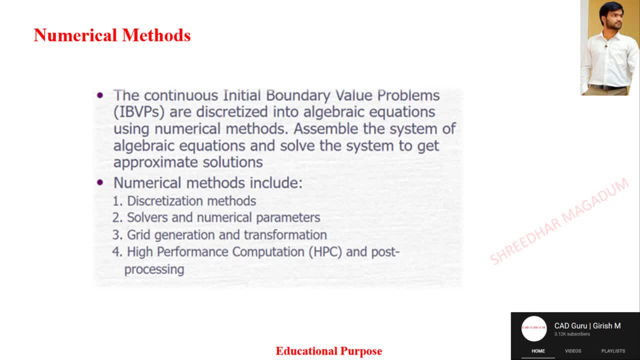 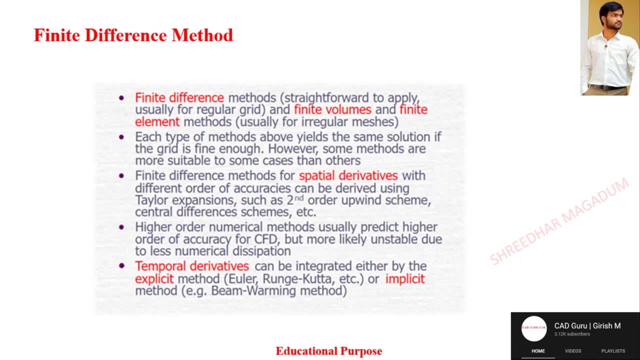 methods. we can consider, that is, discretization method or solvers and numerical parameters. we consider grid generation, transformation and we can consider the post processing with respect to high performance computation, finite difference method, FDM. so in this we'll use the regular grids, okay, and the finite volumes and finite element methods to 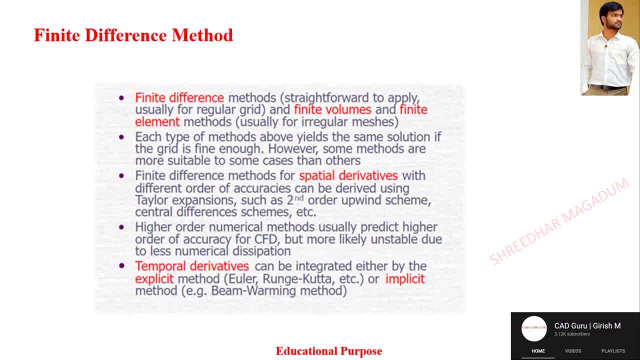 deal with the FDM, so mesh will be irregular. okay, usually we gonna use the second order of wind scheme as well as the Taylor expansions to deal with this kind of FDM. and sometimes we can use the explicit method. so in explicit methods we can use, that is, ELS methods and Rangipunta methods, or for implicit method we can. 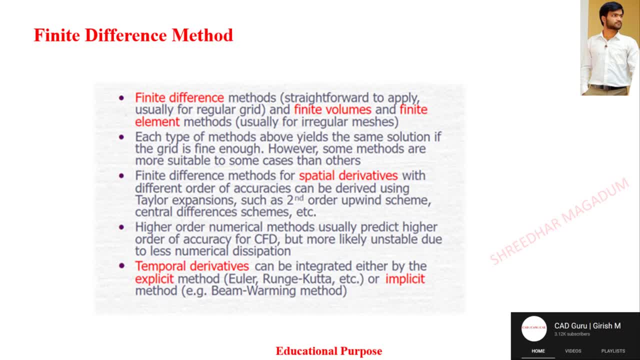 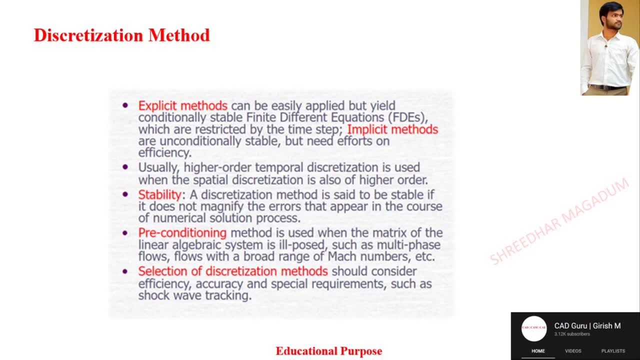 use the V moment method depends upon the requirement. we can just choose the explicit or implicit. okay, if I consider again explicit, here we use the FDM conclusion says that conditionally okay with the time is restricted by the step. okay, implicit methods are unconditionally stable but need more efforts on the efficiency. so 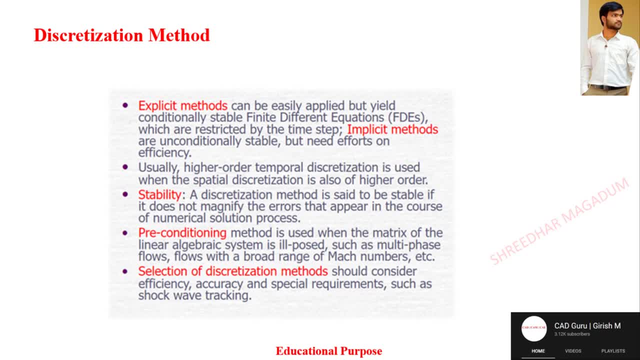 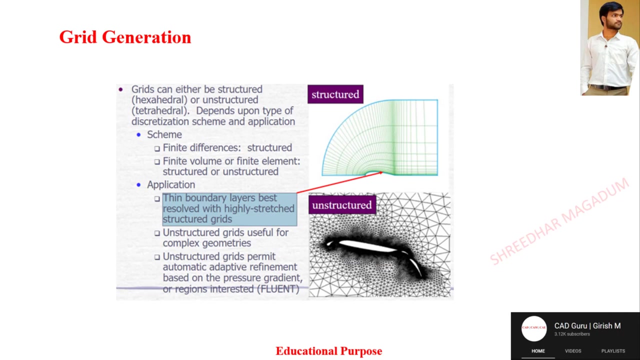 again, you could see a few of the things here: pre-processing conditions and stability and the selection of discretization methods. okay, so if you want to consider the better answers or results or accuracy or the efficiency, we need to use the better mesh generation. so, as you could see, there are structured and unstructured meshes. okay. 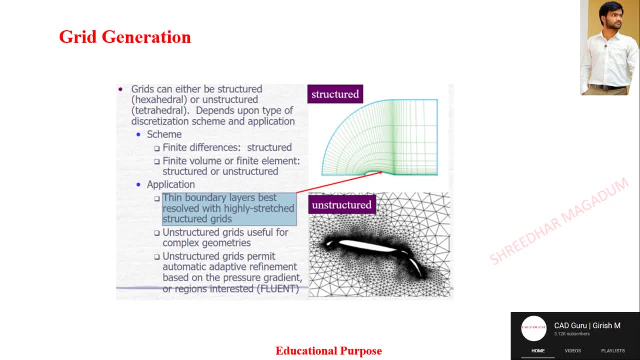 the finite difference method will use the structured mesh into account if I consider the FVM or the finite element, the structured or unstructured, depending upon the accuracy required. okay, so, unstructured mesh will be used for more complex models where the results needed with more accuracy, precision, we can use the unstructured grids. okay so, so, like access fluent will help you with the. 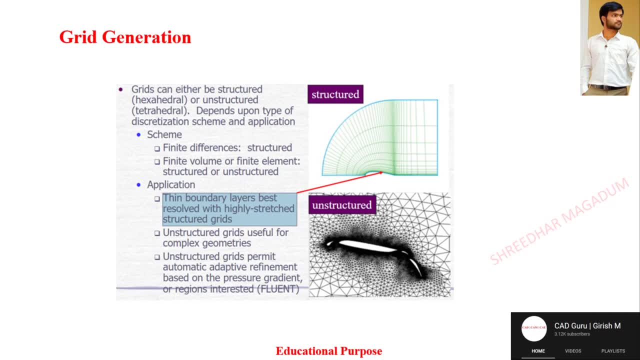 with that, and even we have different solvers in the market to deal with these. okay, so these, these are the two different types of mesh: structure, usually hexahedral, and unstructured is usually tetrahedral. remember that they are very important terms: safety codes, the fluent star, cd, star, ccm, you. 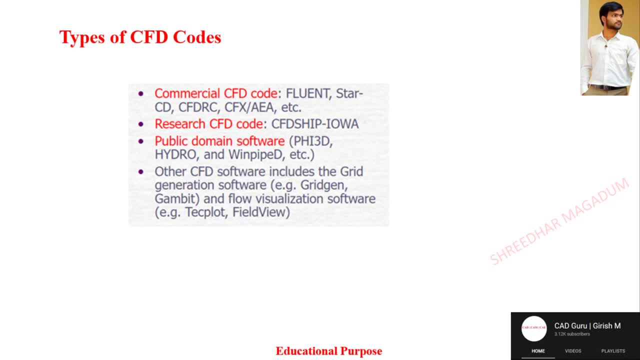 can consider and if I go ahead with the other, safety software software service, like grid generation- they are grid trend, cram, bet and tech plot and feel. fee for the flow visualization: okay, there are different softwares available, so these are the few explanation for that simply process. what exactly will happen? we? 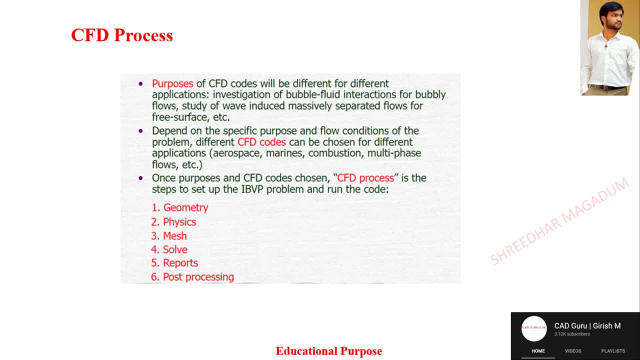 already seen the flow chart. so there we use the geometries and then physics and then mesh it, solve it to put generation and the post processing stages. okay, and purpose, we have seen already. safety codes are as well, we have seen. okay, depending upon the flow conditions and the problems, we'll just go with the. 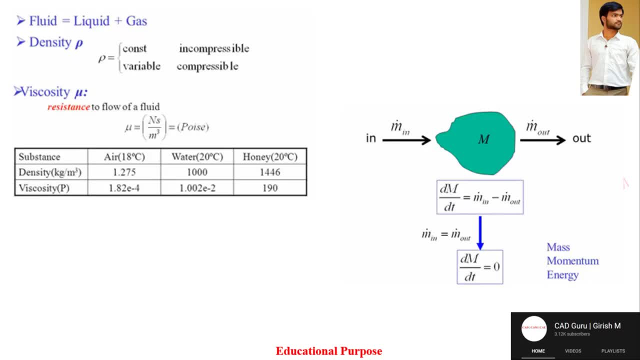 requirement. coming to the density and the viscosity of the substances, that is, air, water and honey. we have taken into account. density of the air is 1.2 and the viscosity and same. for the water thousand and remaining things okay. viscosity is the resistance to the flow. 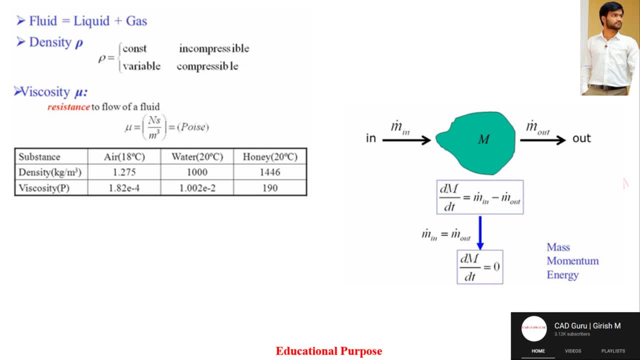 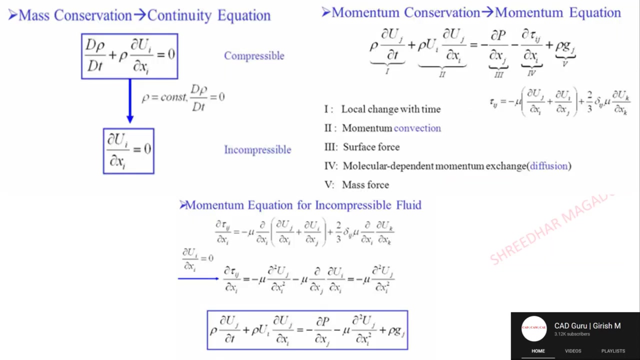 of the fluid. it is measured in poise formula is given density. if I considered constant. if it is, density is constant, incompressible. if it is variable, compressible, okay, this is a momentum, mass moment of energy equation. if the momentum is the mass, conservation takes place here. okay, continuity equation. we 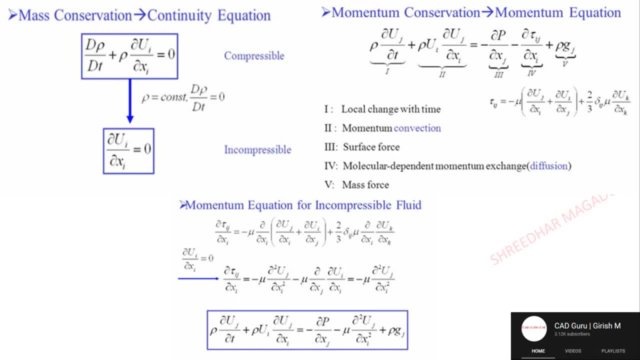 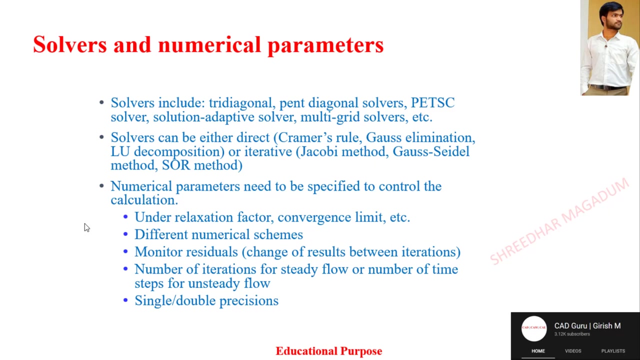 can say that one. so this is the formula for that. if I consider the momentum conservation, that is momentum equation, this is: this is for the incompressible fluid. finally, the solvers and the numerical parameters. solvers include tri-diagonal and pendygonal solvers, and 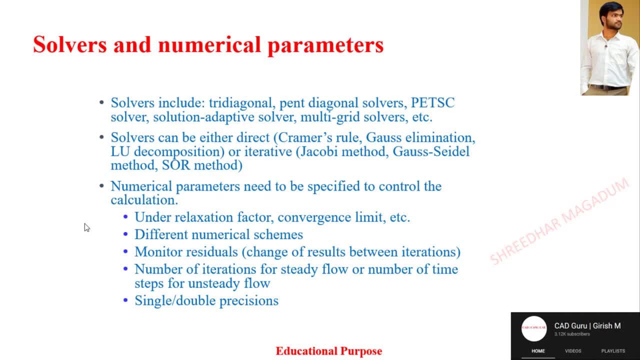 okay, we can even consider the multigrid solvers as well. okay, solvers can be either direct, that is, cramma stool, and the class elimination method. well, we can consider you an LU decomposition. if I consider it, ready method will take the Coddin method into account and each and each of open methods as well, as we saw. 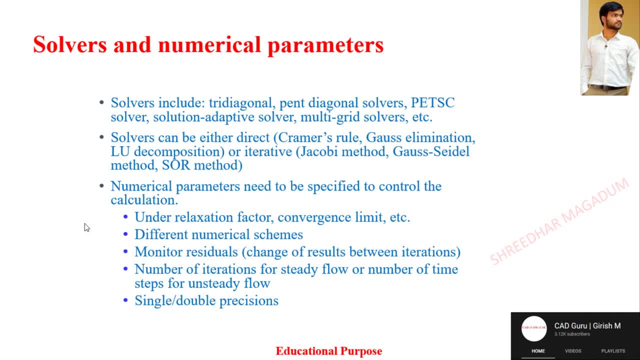 numerical parameters needs to be specified to the control calculations, so these are so large. if you get the results there, we need to consider these residuals like a change of results between the iterations. let's say, if I consider the CDCL coefficient of lift and drag values, so how exactly it is.